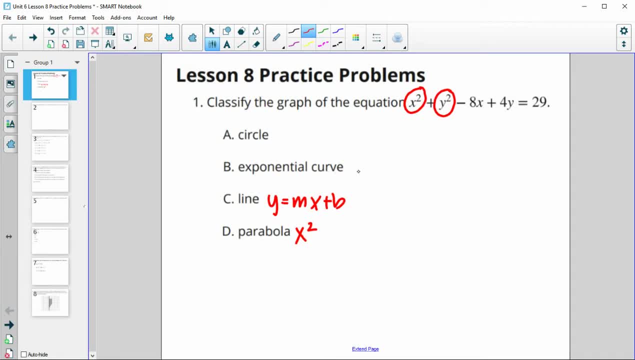 your variable. your x and your y would not be squared Exponential. your variable would be in the exponent. So you would have something like this: e to the x or 2 to the x, But your x would be up in the exponent. So you would have something like this: e to the x or 2 to the x. 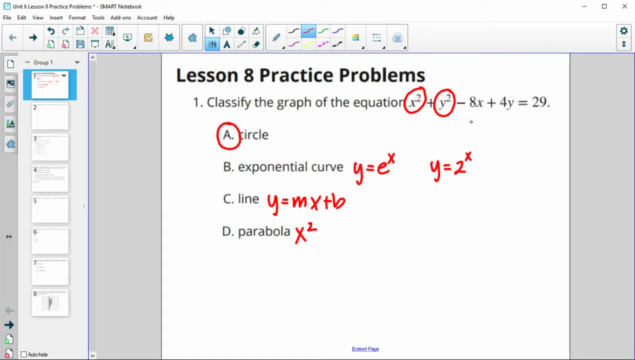 A circle is the one that we've talked about- that has both the x and the y variable being squared. For number two, it says: write an equation that states that the point x- y is the same distance from the point 4, 1 as it is from the x-axis. So this is going to be writing a parabola. 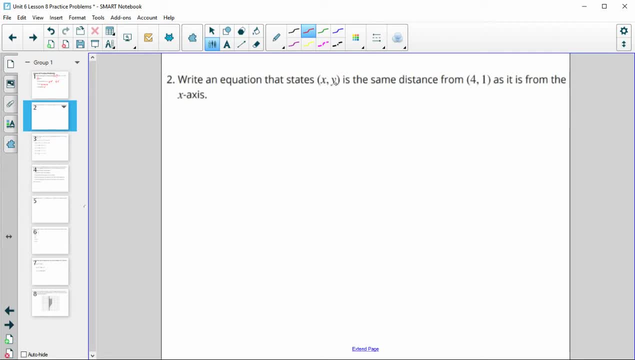 Since a parabola is the same distance from the x-axis, it's going to be writing a parabola, So this is going to be a set of all points, equidistant from a point called the focus and then from the line, the directrix. So here's your focus and here's your. 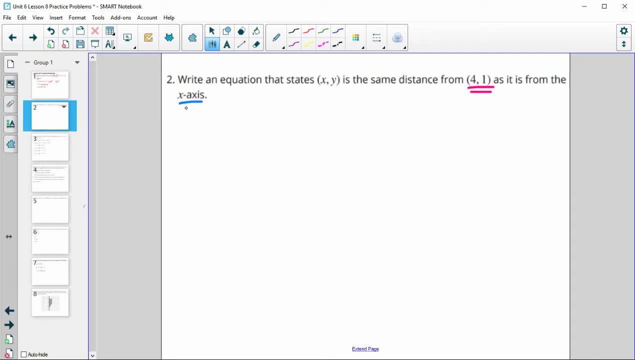 line, the directrix. So this one I like to write as a: y equals line. So the x-axis is the line y equals zero. So if we remember, when we're writing equations of parabolas, the distance to the y-axis is the same as to the point. So that will be on this side of the equation. We'll do y minus. 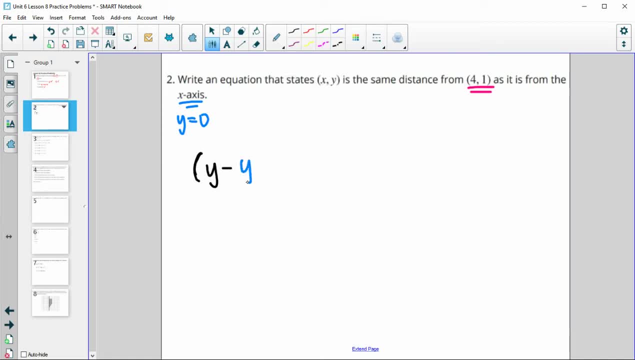 the y-coordinate of your directrix. I'm just going to put y sub d, d meaning directrix, So that'll be our distance to our directrix, And then we will do the Pythagorean theorem to figure out how far the point is from the focus. And so this will be x. 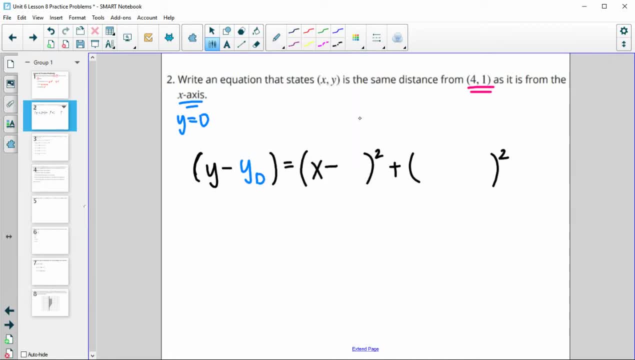 minus the x-coordinate of your focus, And then the y-coordinate minus the y-coordinate of your focus, And that's going to represent the horizontal and the vertical distance between the two points. So here would be your point, x, y And here would be your point. 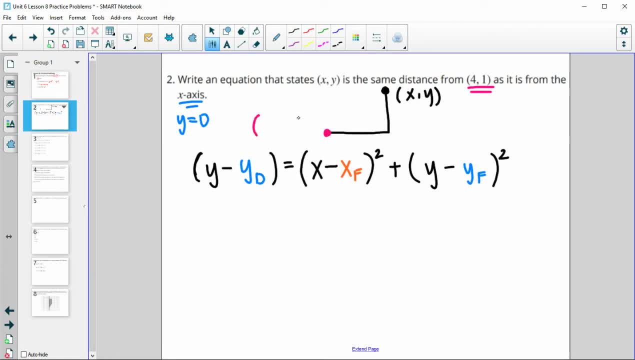 the focus. okay, so this would be your y of your focus and your y of your focus. And then the distance here, okay, is from the point to that directrix line, So y minus the directrix y-coordinate, So in this case we have y-connection d. 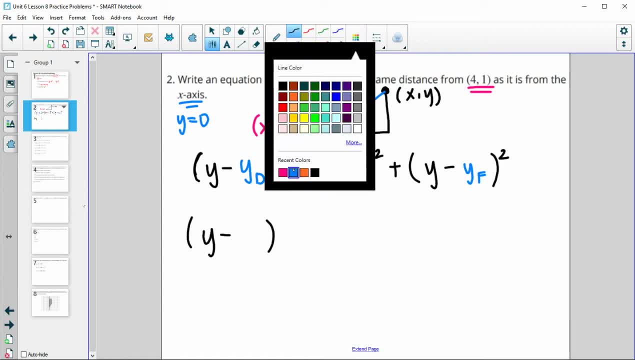 y minus 0,. since the directrix is 0, equals x minus the x-coordinate of the focus. So the x-coordinate of the focus is 4, plus y, minus the y-coordinate of the focus, And the y-coordinate of the focus is 1.. 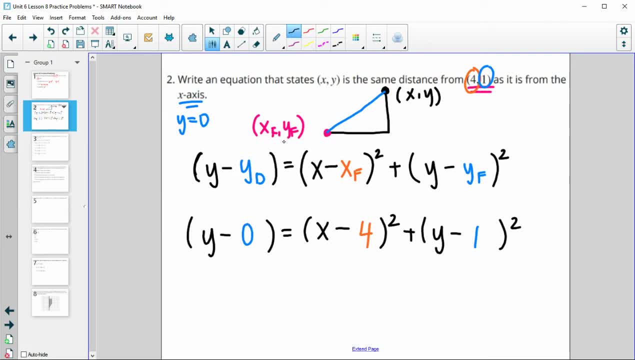 So that would be our parabola. Oops, I forgot This should be squared. So then you could clean it up just by saying that this is just going to be y squared, And then this will just stay: x minus 4 squared and y minus 1 squared. 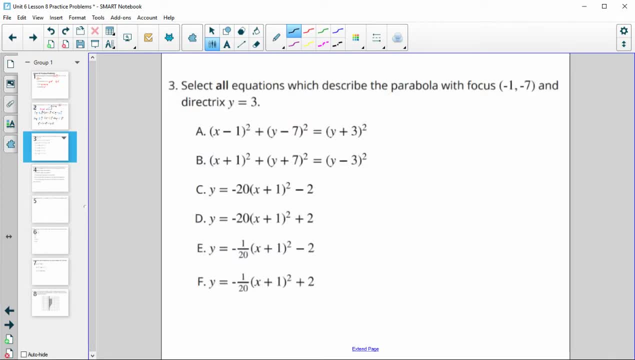 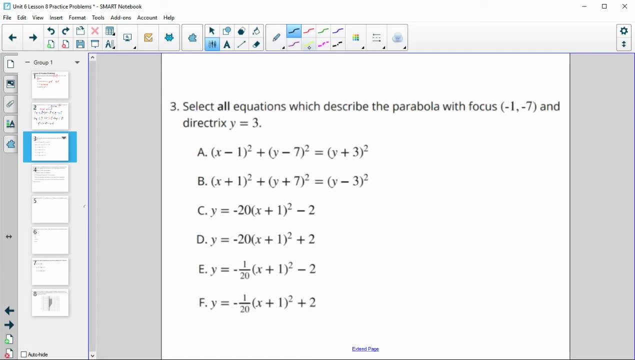 Number three: select all equations that describe a parabola with a focus of negative 1,, 7, and a directrix, And then you can use the directrix of y equals 3.. So first off, let's just look at writing the equation of the parabola. 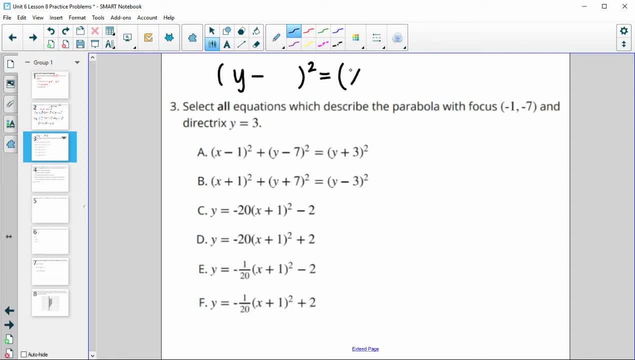 So the distance to the directrix will equal the distance between the points from the point to the focus. So the distance to the directrix is y minus the y-coordinate of the directrix. Then the distance between the points will be the subtraction of the x's. 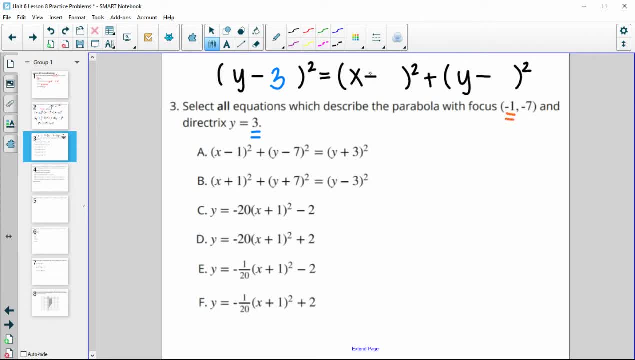 So we'll do x minus the x-coordinate of our focus, So y minus negative 1, we'll turn that to plus 1 squared. And then y minus the y-coordinate of the focus, So y minus negative 7, we'll turn that to positive 7.. 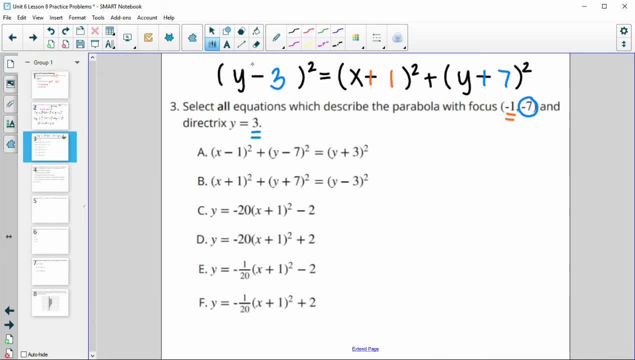 So that's our parabola formula that we've kind of been looking at. So now we can look at these first two that are written in that form And we see that this one has x minus 1 instead of x plus 1.. 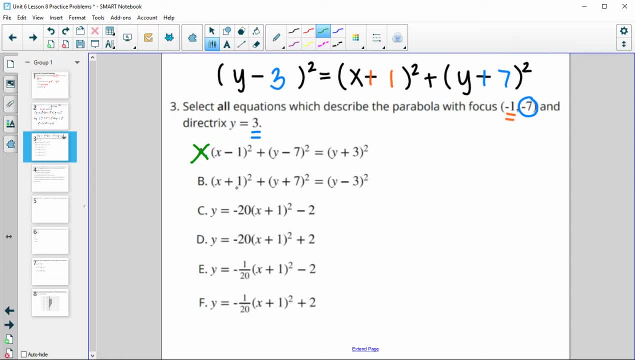 So that is not correct. This one has the x plus 1 squared, the y plus 7 squared, and it's equal to y minus 3 squared. So this is good, Then. what they've done is taken this kind of directrix form here. 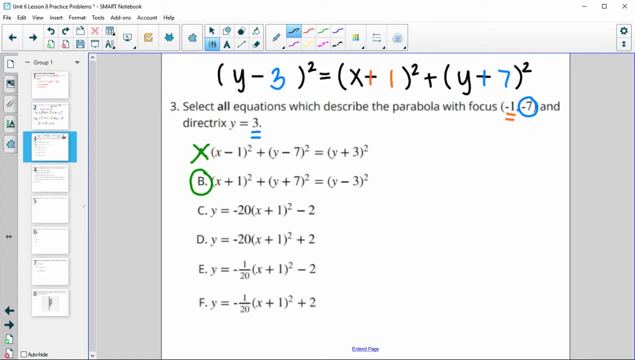 and they've written it in vertex form. So they've multiplied out this y minus 3 squared. Okay, so a binomial squared. we know that's going to be y squared minus 6y plus 9.. Now all of these still have the x plus 1 squared. 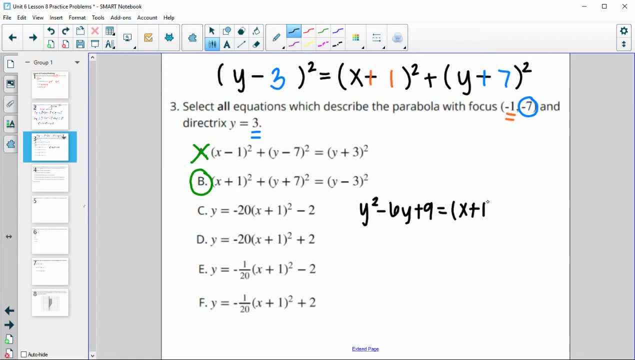 So we're going to leave that, We're not going to touch that, So we're just going to leave it as x plus 1 squared, And then we'll multiply out this y plus 7.. So that will be y squared plus 14y. 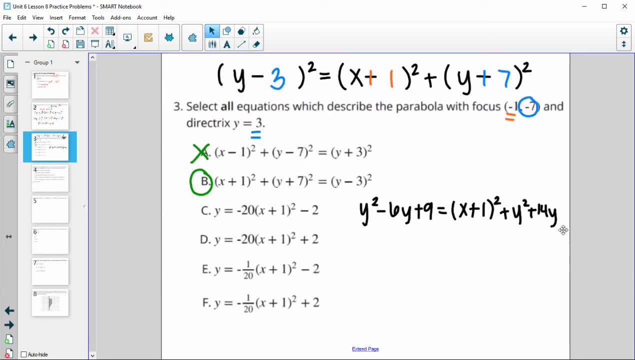 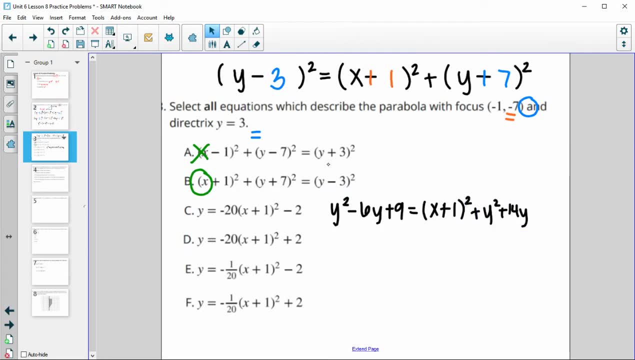 Let me move this over a little bit here. Whoops, I don't know if it's going to. let me, Let's see. Okay, let me move this over just a little bit so we have some more room. So that's going to be y squared plus 14y plus 49.. 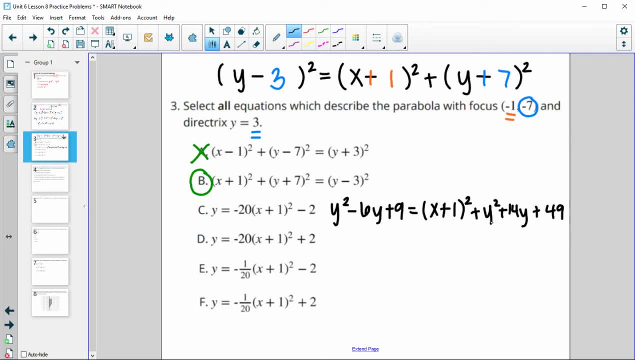 So now they're going to bring all of the y terms to the left, so let's subtract this y squared from both sides. We're also going to subtract this 14y from both sides, And I just lined it up under its like terms. 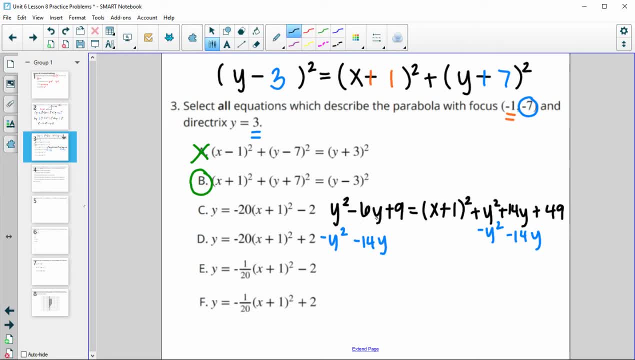 So y squared minus y squared is 0.. 6y minus 14y is negative 20y and we have that plus 9.. And then 8y, So that equals x plus 1 squared. Y squared minus y squared is 0.. 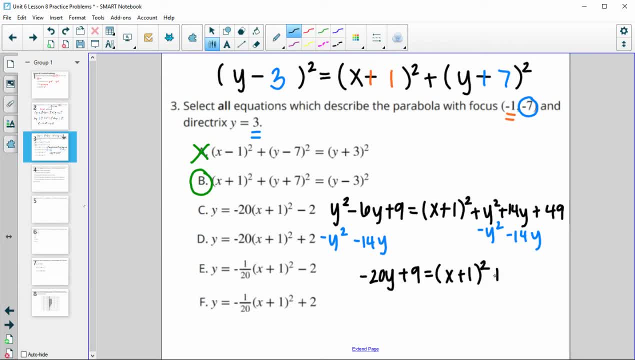 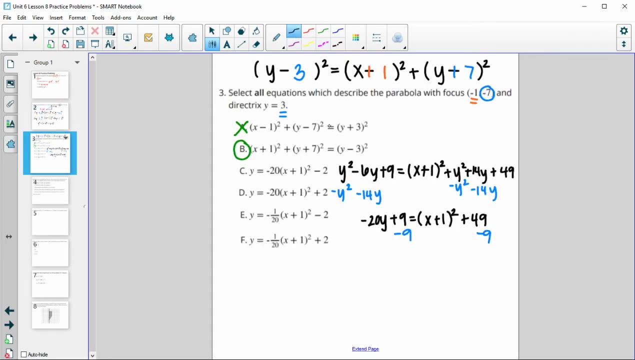 14y minus 14y is 0, and we have that plus 49.. So then we'll subtract 9 from both sides, So we can get those constant numbers together. So then we end up with negative 20y. 9 minus 9 equals 9.. 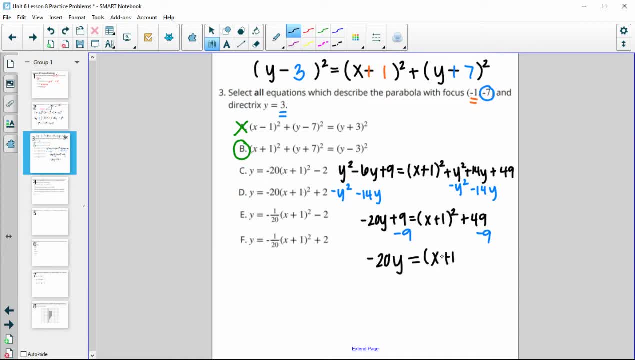 is 0, x plus 1, squared 49 minus 9 is 40. So then we'll divide by negative 20 to get the y by itself, and you'll do that to each term on the right hand side. So negative 20y divided by negative 20 is: 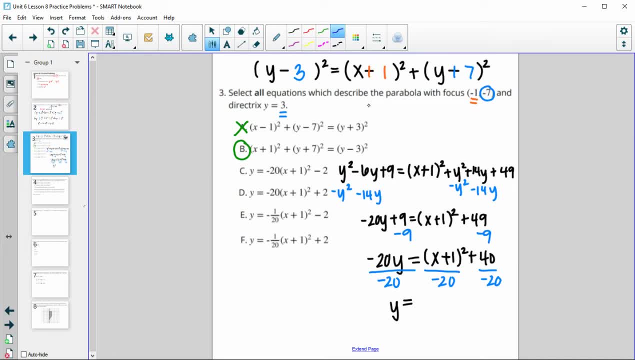 just 1y, And then for this one, x plus 1 squared divided by negative 20, I'm going to think of this as having a 1 up top. So 1 divided by negative 20 is negative 1 20th, And then x plus 1 squared. 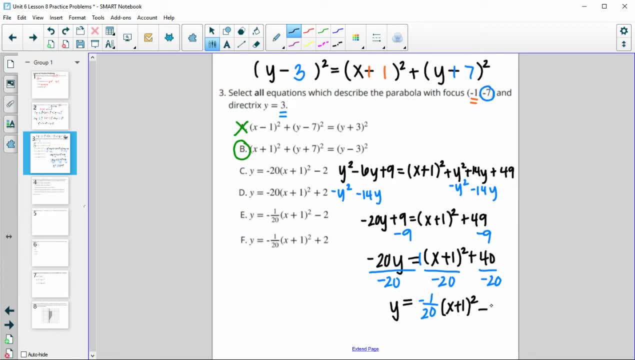 40 divided by negative 20 is negative 2.. And then we can kind of do that to each term on the right hand side And then we can kind of match these up So we see that it has a negative 2, so it can't be these: 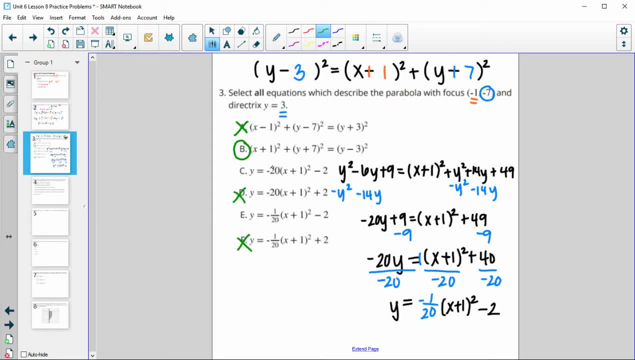 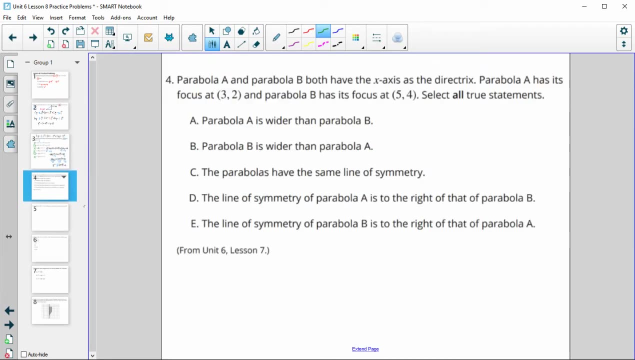 ones with the plus 2s. This one has negative 20, okay, which is not what we want. We had negative 1, 20th- Okay. number four says parabola A and parabola B. both have the x-axis as a directrix. 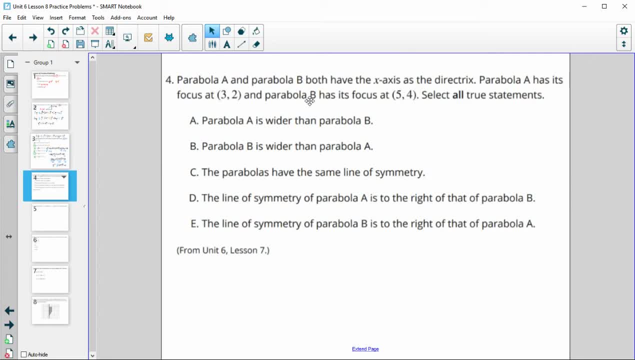 Parabola A has its focus at 3x. Parabola B has its focus at 5x. Parabola B has its focus at 5x. Parabola B has its focus at 5x. Select all true statements. 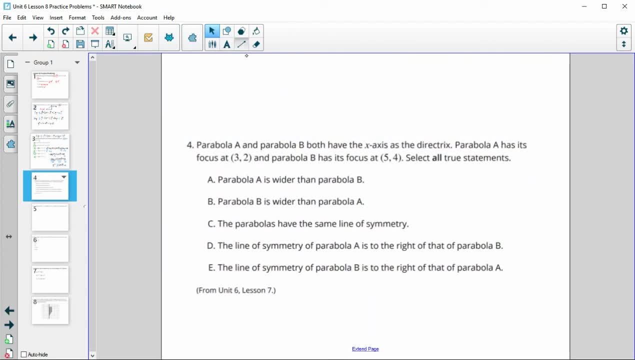 So I like to draw pictures of these to help. So we'll draw parabola A here. Whoops. So I'm just going to draw the xy-axis here, And this one says that parabola A has a focus of 3x. 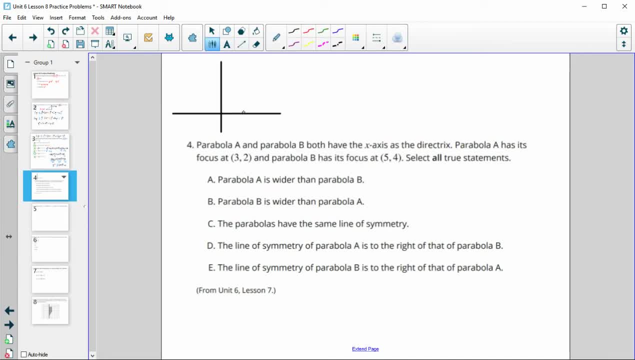 Parabola A has a focus of 3x. Okay, so it has a focus of 3x, So we'll just put a point here. So here's our focus, And then it has a directrix of the x-axis. 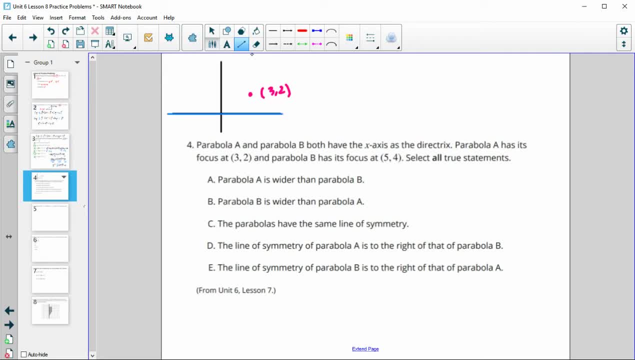 And so that's this line right here, And I also like to write this as the y-line that it is. So this is: y equals 0.. Then, and that's parabola A, Then parabola B Has a focus of 5, 4.. 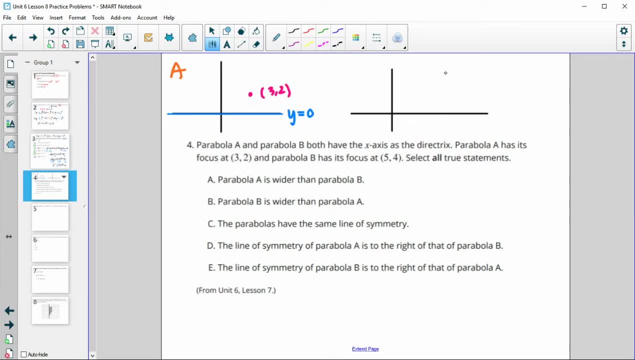 Okay, so 5, 4.. And then a directrix of the x-axis again, Which again is the line y equals 0. So let's see if we can come up with which statements are true here. So parabola: A is wider than B or B is wider than A. 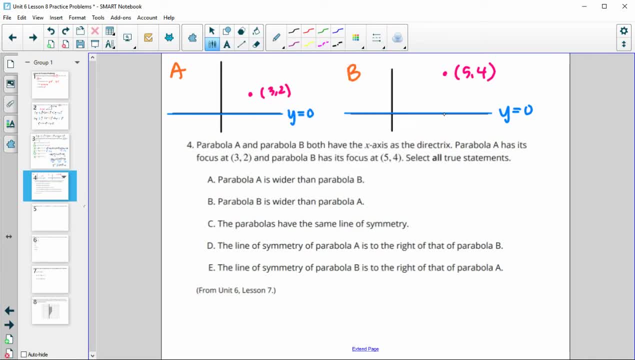 So, remember, the further the focus is from the directrix, the wider the equation is, or the wider the parabola is. So this parabola here is going to be narrower than this one, since the distance, Since the distance here. okay, the distance from this focus to the directrix is four units and this one is two. 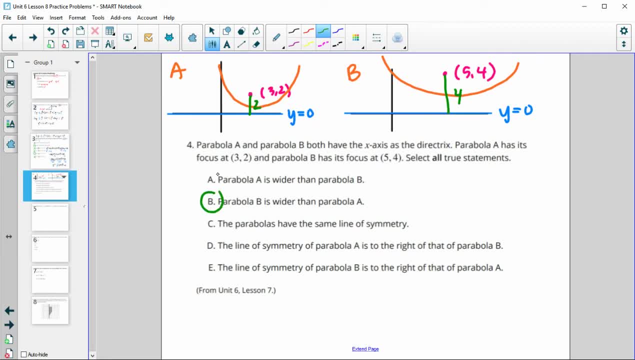 So B's parabola will be wider, So B is wider than A. The parabolas have the same line of symmetry, So this is asking, basically, if they are at the same X coordinate, Because the line of symmetry is going to cut right through the focus. 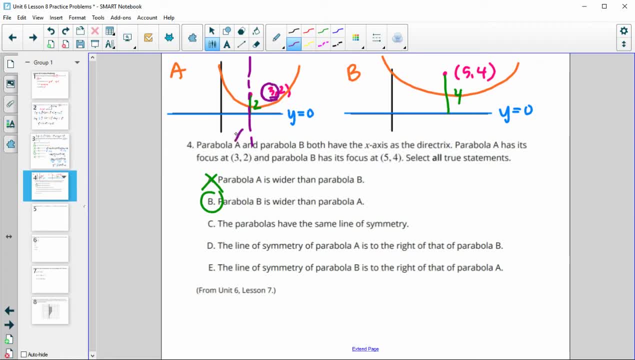 So this one has a line of symmetry of X equals three. This one's line of symmetry is X equals five. So they do not have the same line of symmetry. The line of symmetry for parabola A is to the right of B or B is to the right of A. 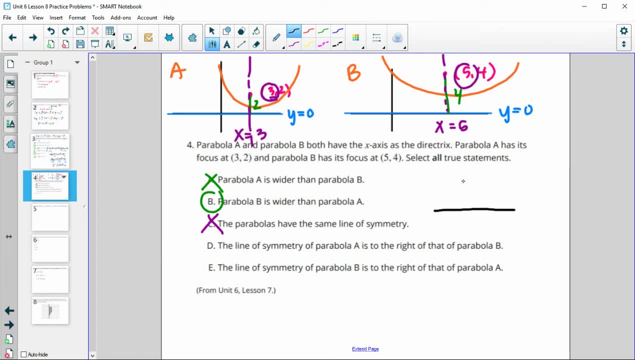 So the line of symmetry. so let me just draw it over here. So the line of symmetry for A is at: X, equals three, right? So this is A's line of symmetry, and B's line of symmetry is at: X, equals five. So which one is to the right? 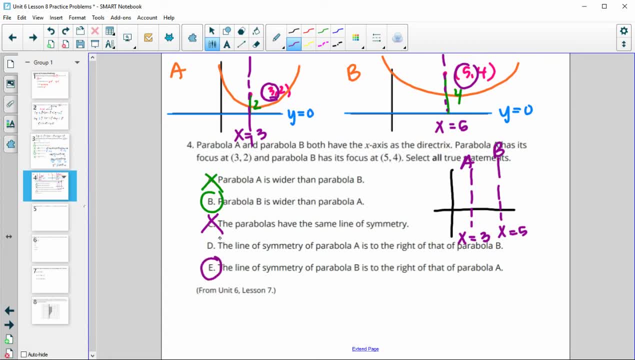 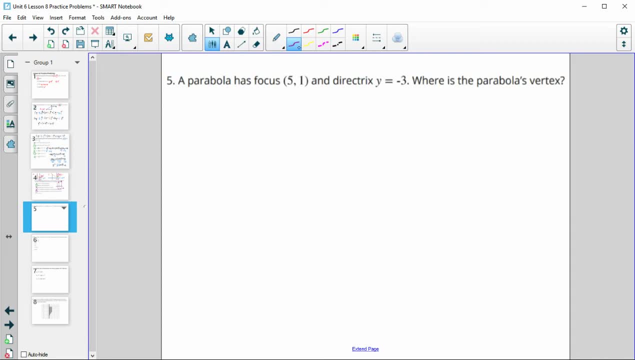 So B is to the right of A, Number five. parabola A has a focus of five negative or sorry five units. So B is to the right of B, Number five. parabola A has a focus of five negative or sorry five units. 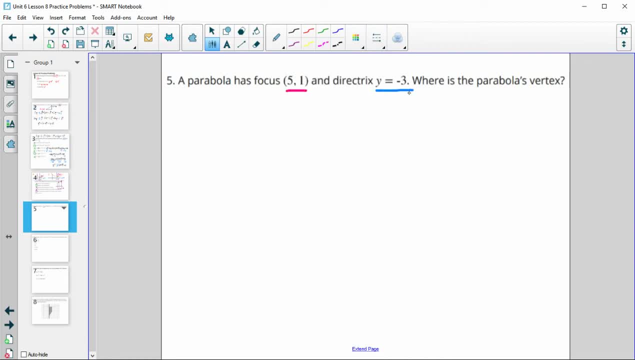 So B is to the right of B, Number five, parabola A has a focus of five negative- or sorry five- units And a directrix of Y equals negative three. What's the vertex? So remember, the vertex is directly between the focus and the directrix. 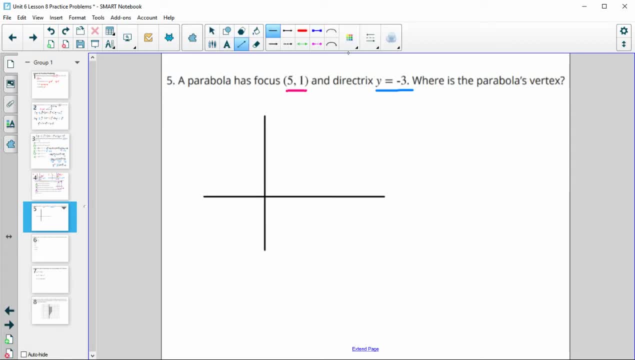 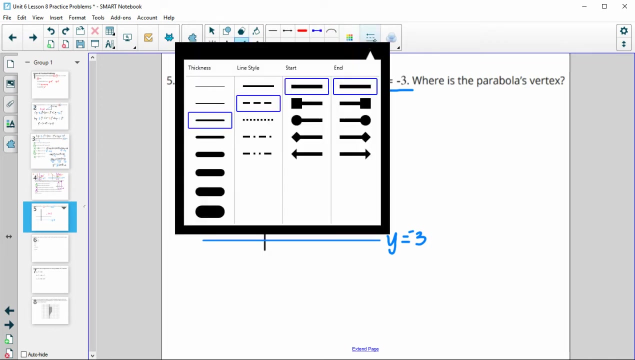 So let's just draw a quick sketch here. So the directrix is down at Y equals negative three And the focus Is at five one. So the vertex is going to be directly between these. It's also going to be on the same X line. 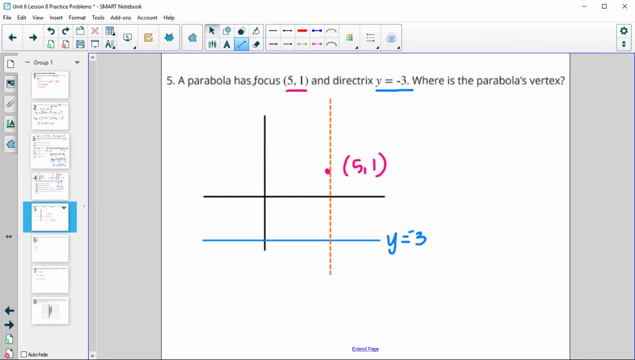 So it's going to be on this same vertical line here, which we know. So we know the X coordinate will be the same. So the X coordinate here Is five. So we want to figure out the Y coordinate that's in the middle here. 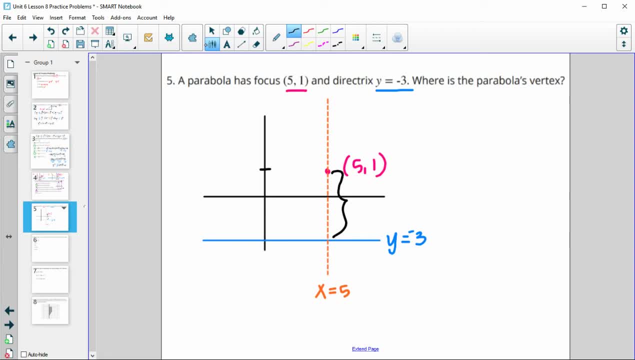 Okay, so this one's at one And this one's at negative three. So we could kind of draw these on here. So that's one negative, one, negative two, negative three, And you could find the middle that way. So then the direct middle between these: 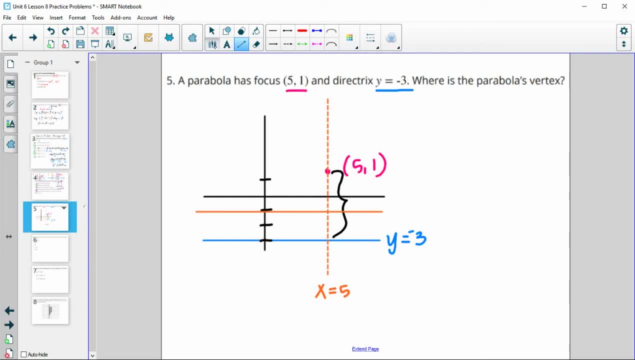 Would be at negative one. So you could do it that way And that would give you the vertex. So this is: Y equals negative one. This would give you the vertex of five, negative one. Okay, you can also. So remember, we know that the X coordinate is the same as the focus. 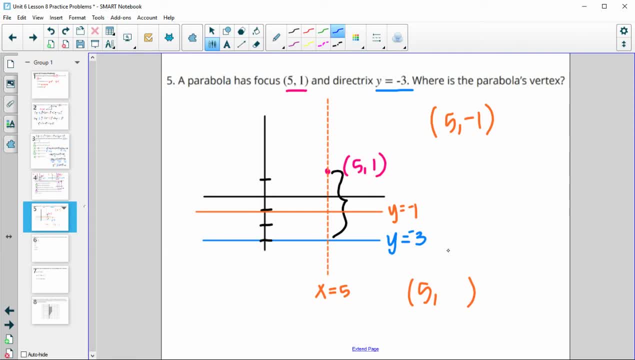 Okay, so we knew this was going to be five. So again we're looking for this Y value here And we want it to be in the middle of one and negative three. So middle Middle is just average. So you can take and add one and negative three and divide by two. 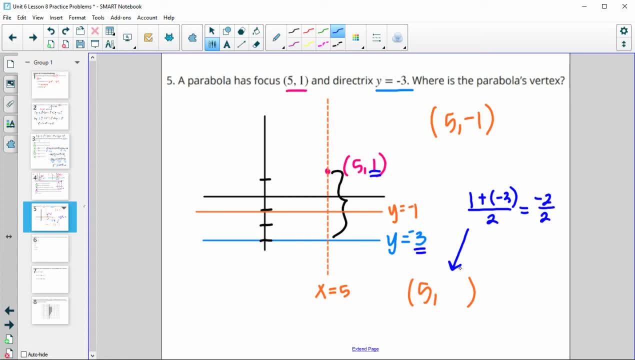 So one plus negative three is negative two, Divided by negative two is negative one. That's another way you could get it. Okay, number six. So select the value needed in the box in order for the expression to be a perfect square trinomial. 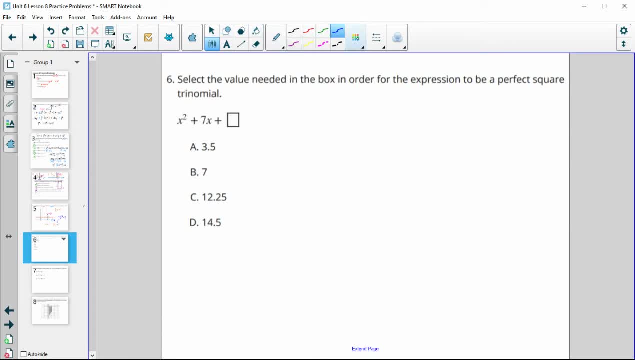 So, remember, this is where we take the middle term And we divide it by two. So in this case we'll get 3.5.. And then we square this, And 3.5 squared is 12.25.. Number seven: rewrite the expression as the product of two factors. 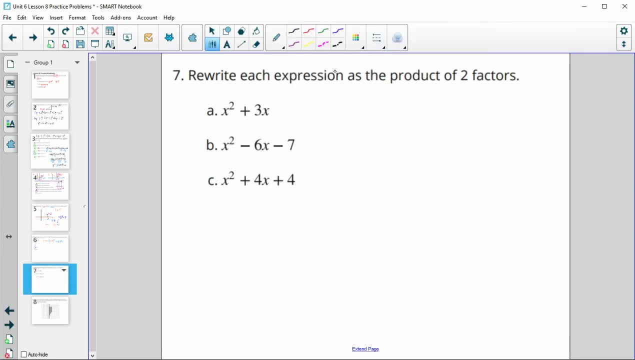 So in this first one we just have a common factor of X that we can take out. So we'll factor that out. So after taking the X out, So X squared, divided by X, we're left with X. 3X divided by X, we're left with three. 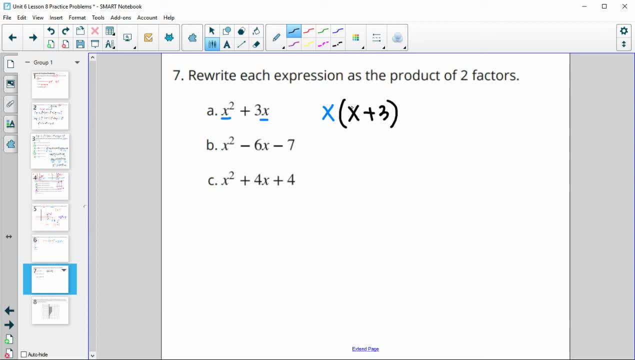 Remember, you can look at this and make sure that when you distribute the X, that it equals back to this. So X times X is X squared. X times three is 3X, Factoring a trinomial. Now, this is not a binomial squared. 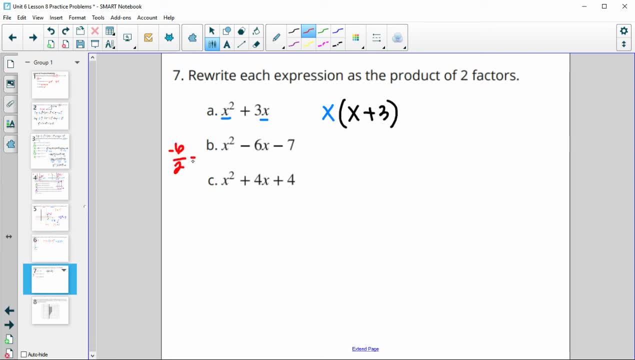 We can tell, because negative six divided by two is negative three And negative three squared is nine. So this is not like one of the patterns that we've been using. So we want to look for the numbers that will multiply to negative seven. those will go in here. 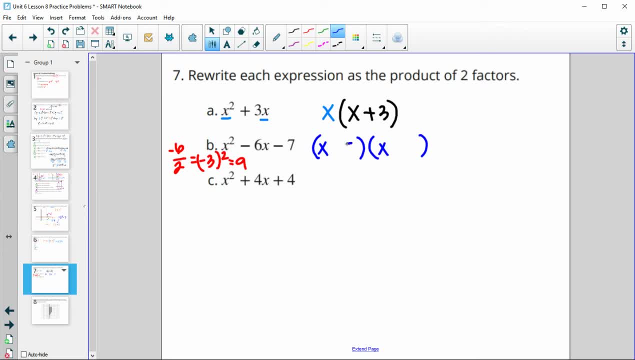 and they have to add to negative six. Okay, so what numbers? and seven is prime, so it's got to be seven and one. So what multiplies to negative seven? So either seven times negative one, or negative seven times positive one. 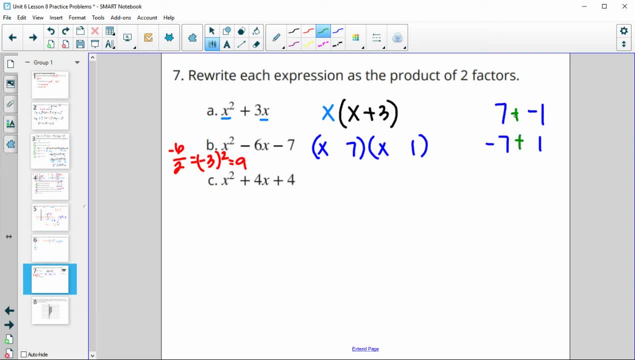 And then we want to find the ones that add to negative six. So seven and negative one adds to positive six. negative seven adds to negative six. Negative seven and negative one adds to negative six. So we want this to be negative seven and positive one. 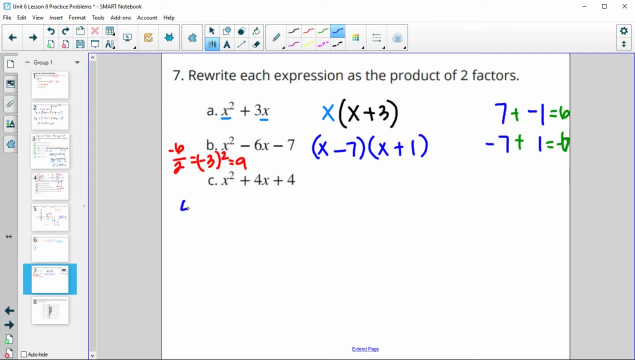 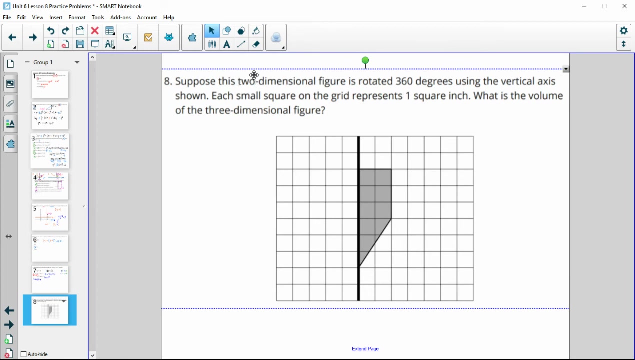 This next one: four divided by two is two, and two squared is four. So we know, this is one of our perfect square trinomials. So this is X plus two squared, And then number eight. so suppose this two-dimensional figure. 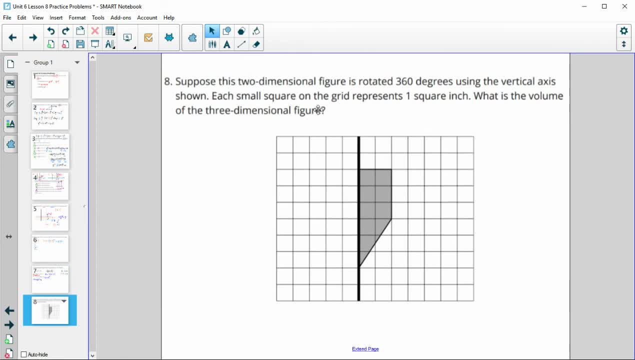 is rotated around the vertical axis. Each small square grid represents one square inch. What's the volume of the solid that's created? So if we spin this around, okay, so if we spin this around, okay, this is going to create a circular motion here, right? 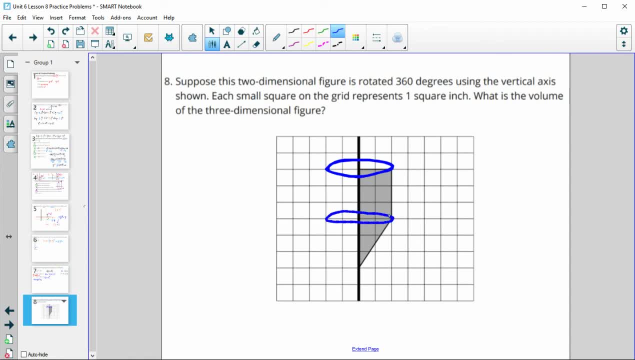 And we've got this circular motion here, Okay, connected, And then this bottom part will connect here. So we've got basically a cone on the- or sorry, a cone on the bottom. So this bottom piece makes a cone as it spins around, right? 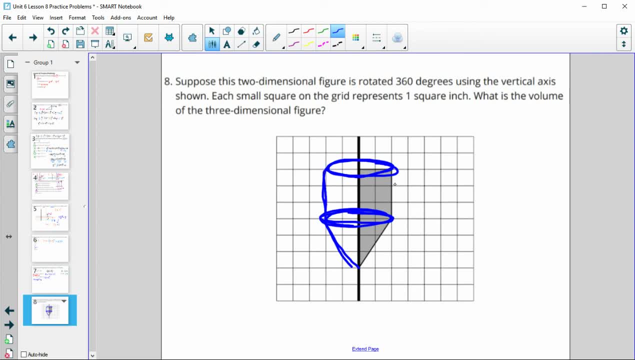 We get this cone And then this top part gives us a cylinder. So the radius of this circle here is two, The height here is three. So when we find the volume of a cylinder, it's going to be the area of the base times the height. 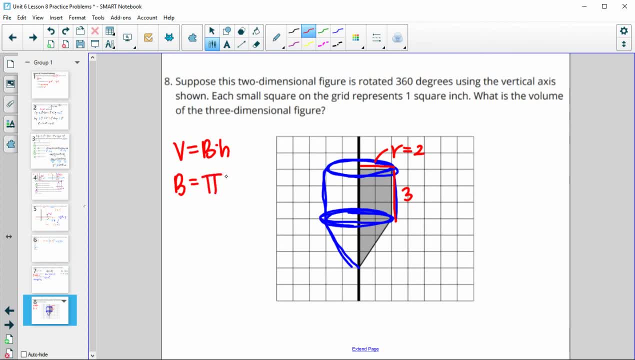 The area of the base. so the base is a circle. So pi times the radius, which is two squared. Two squared is four. So I'll just write the area as four pi for that base And then remember the height of that cylinder is three. 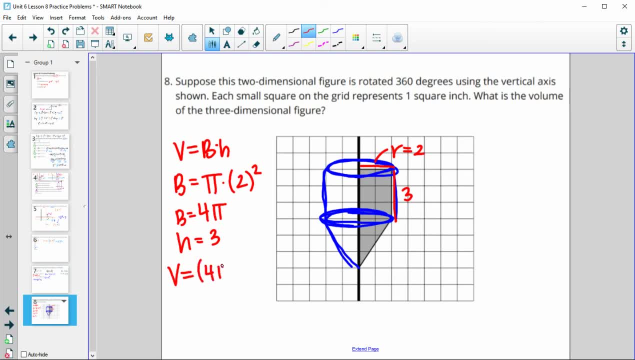 So the volume here is going to be the area of the base four pi Times the height three. So the volume of the top part is going to be 12 pi. Then we can find the volume of this bottom part, so of the cone. 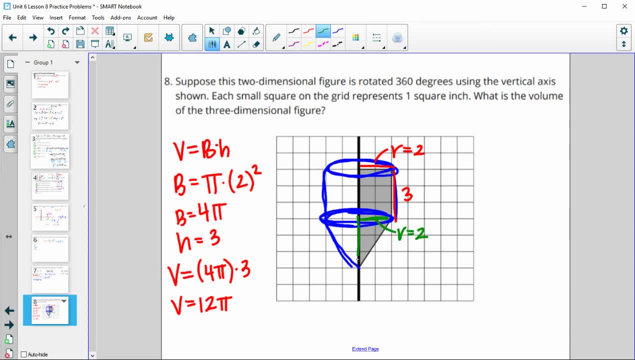 So, remember, this radius is still two, And now we can look at the height. here is also three, So it's a cone with the same base and the same height. So it's just going to be a third of this Because, remember, volume is equal to area.